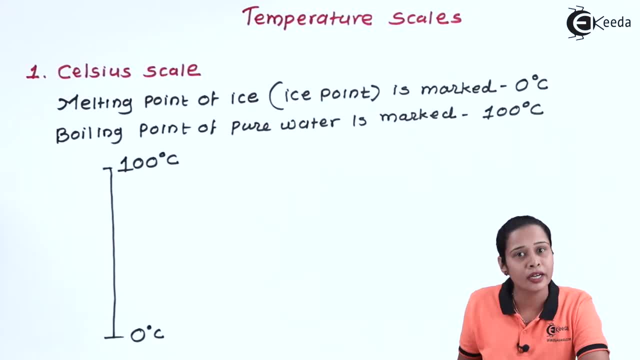 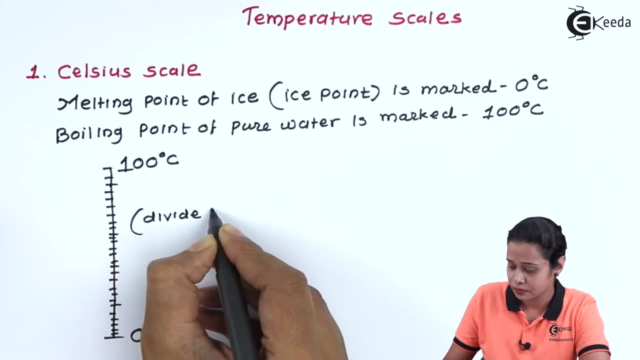 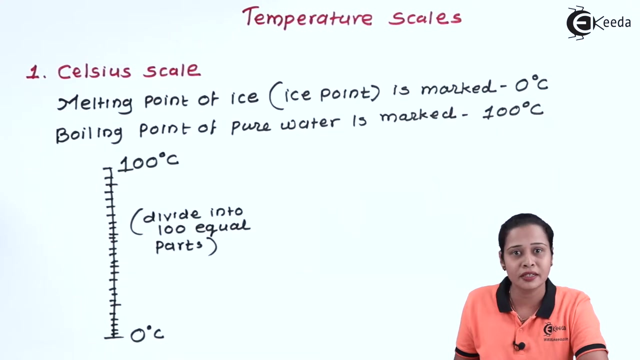 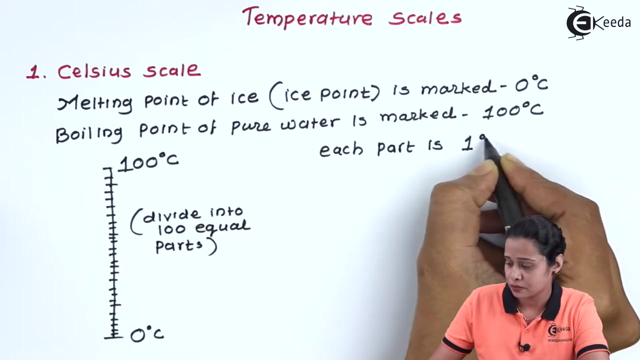 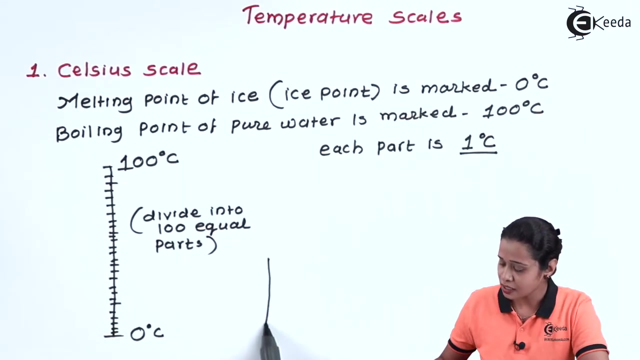 Now this is divided into 100 equal parts. So the scale is divided into 100 equal parts. Now each part is considered as 1 degree Celsius. Now, here we can say: each part is 1 degree Celsius. Now, here we can say: each part is 1 degree Celsius. 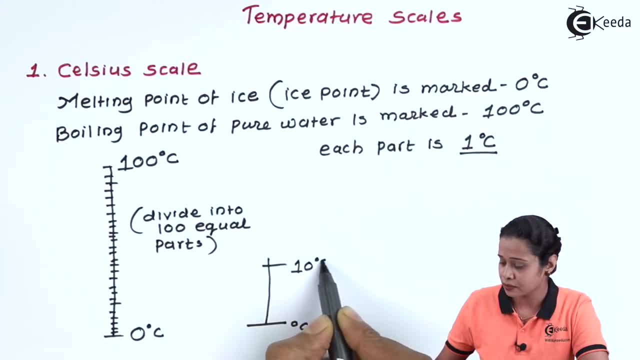 And 1st one is 10 degree. then that is again divided into the 10 equal parts, So the smallest part, this one, will be 1 degree Celsius. So this scale is generally used for the scientific use. So this is about the Celsius scale. 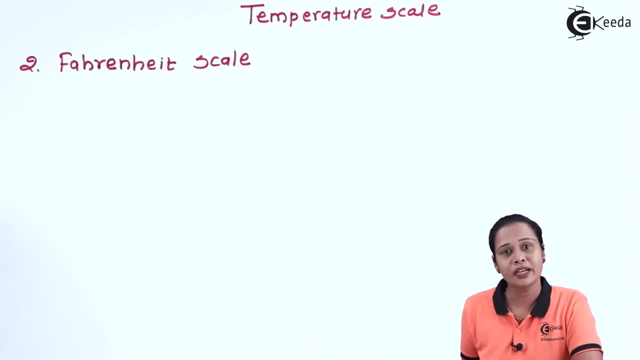 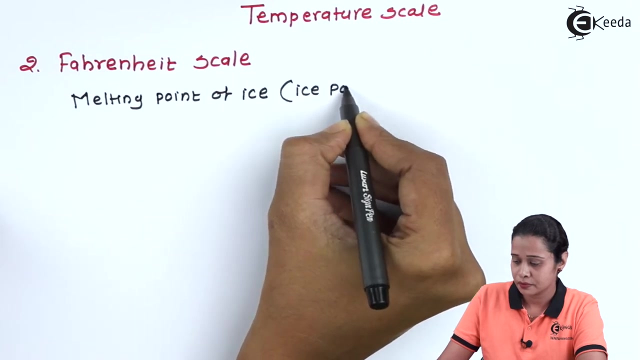 The second one is Fahrenheit scale. Fahrenheit scale is the a herbaceous. The Fahrenheit scale is the a herbaceous. The Fahrenheit scale is the, a herbaceous designed by scientist Fahrenheit. that is why it is called as Fahrenheit scale. Now, in this scale we have 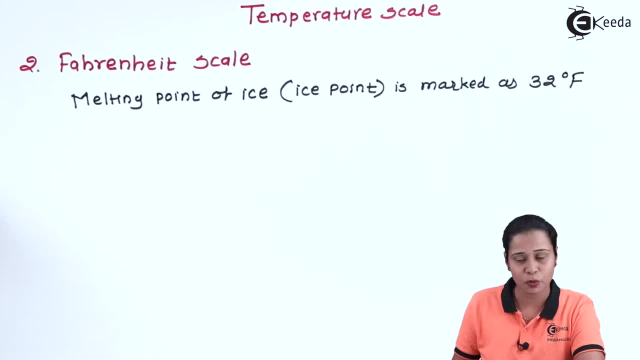 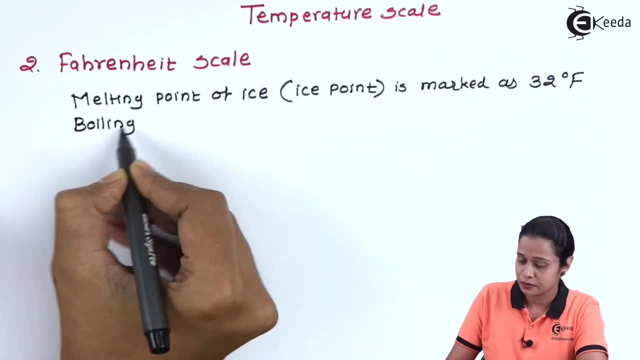 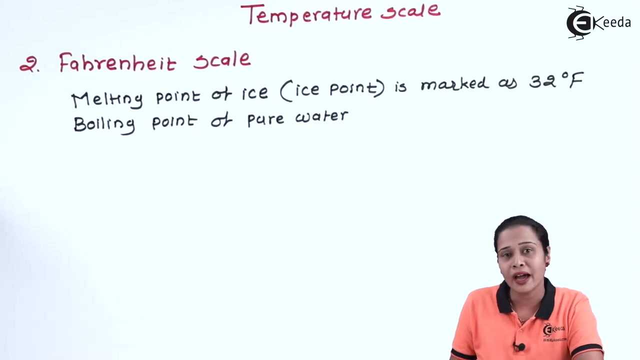 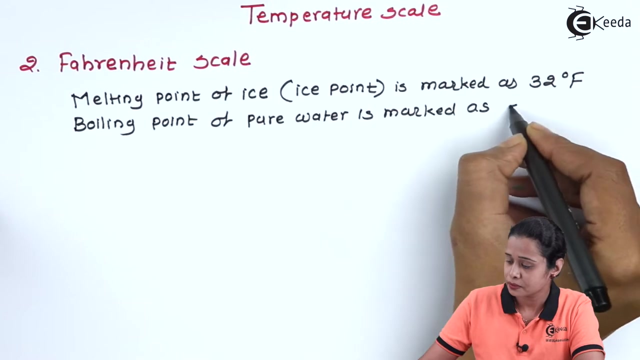 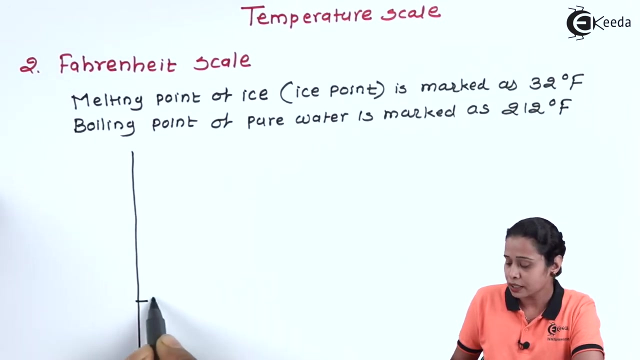 the melting point of ice- this is also called as ice point- is marked as 32 Fahrenheit and boiling point of pure water at constant atmospheric condition is marked as 212 degree Fahrenheit's. now the scale. suppose it is starting from 0, but the 32 Fahrenheit's 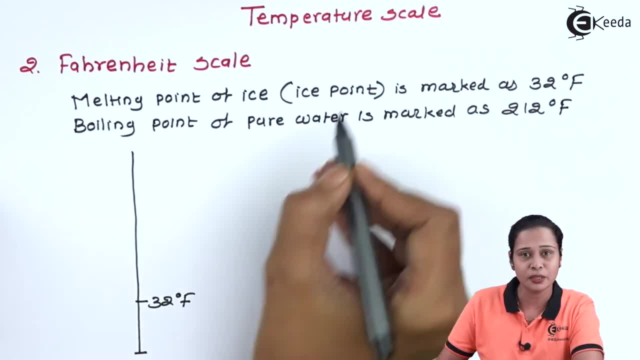 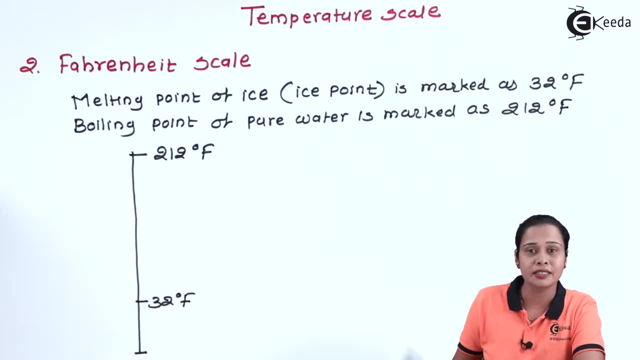 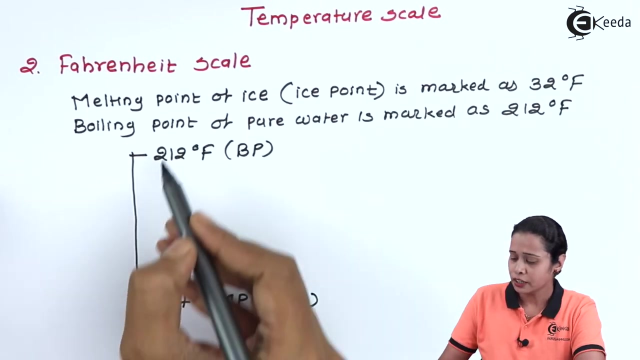 is marked as here the ice point and we have here 212 degree Fahrenheit's, that is considered as a boiling point of water. So we will write here: this is the boiling point of the water and here we can write melting point of ice. Now, if I do, this means 212 minus 32 Fahrenheit's is equal to 0.. 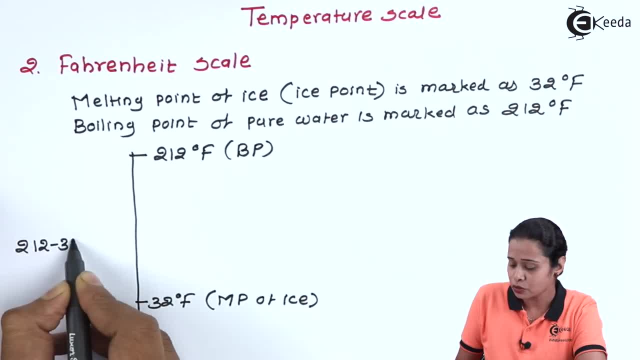 So this is the melting point of water. So we have here 212 degrees Fahrenheit's. So we have here 212 degrees Fahrenheit's. that is considered as a boiling point of water. So if you label now you get 312 degrees Fahrenheit's as 3 て²F is equal to 3 tenía. 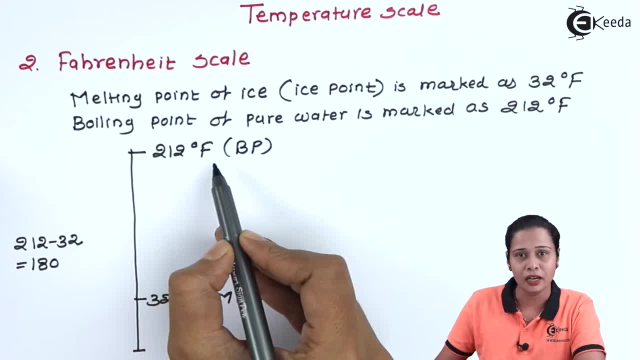 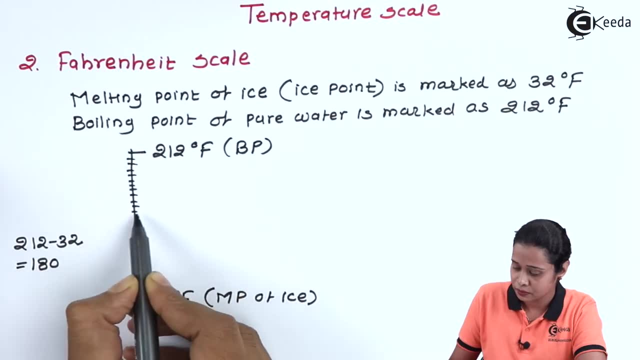 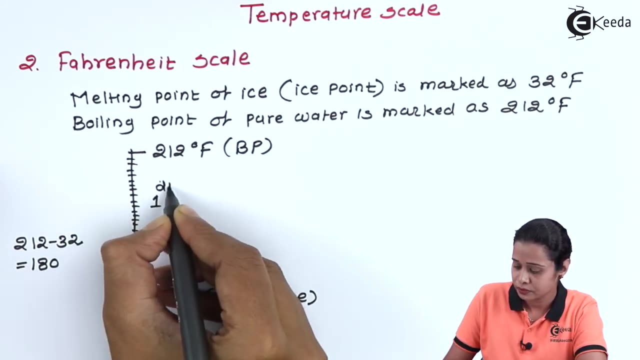 integrate one eighty. So here this 32 to 212 is again divided into 180 equal parts. so let us say this is divided into 3, So let us see what happens now. So it is 12 thousand degrees Fahrenheit's, so in temperature we have 62 degrees Fahrenheit's. 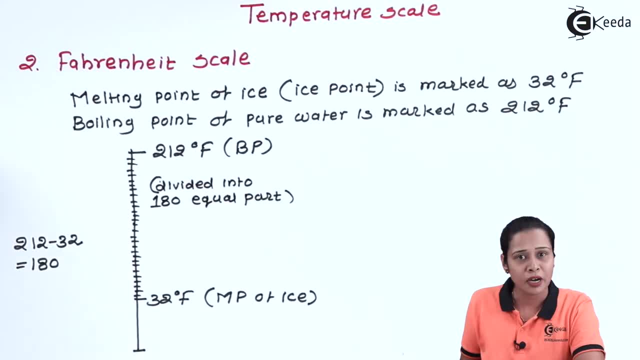 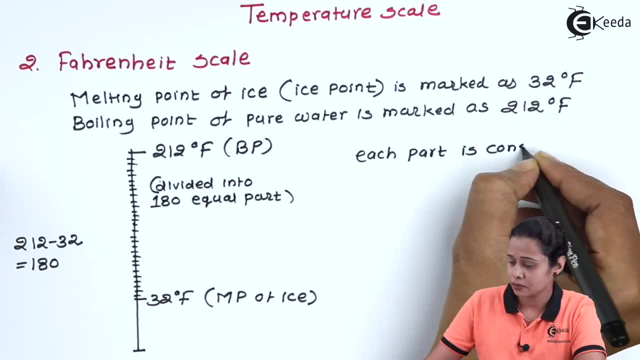 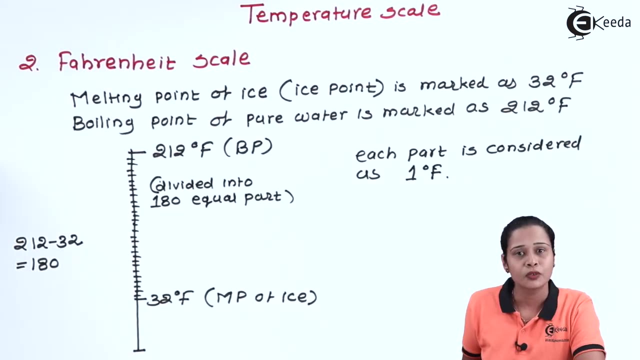 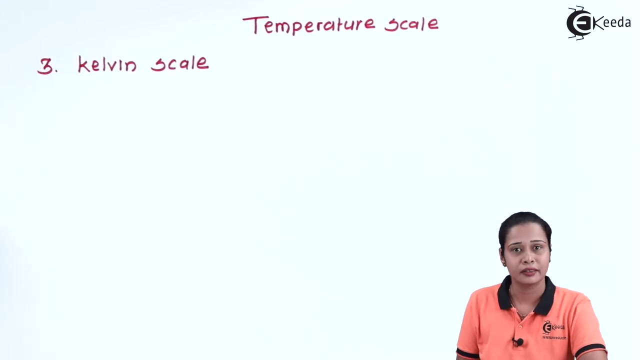 so here 32 Fahrenheit equal to 38. And here each part is considered as 1 Fahrenheit. This type of scale is generally used for the medical purposes. So this is about Fahrenheit scale. Now let us start with third scale, that is, the Kelvin scale. 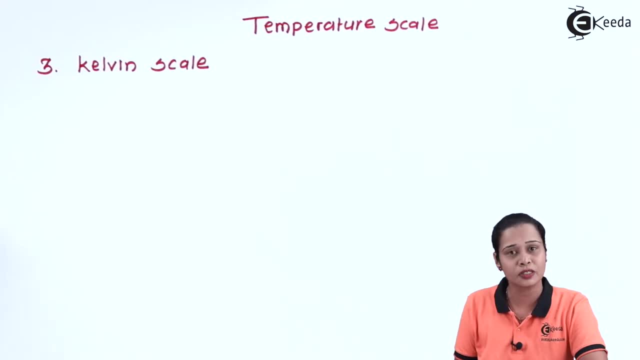 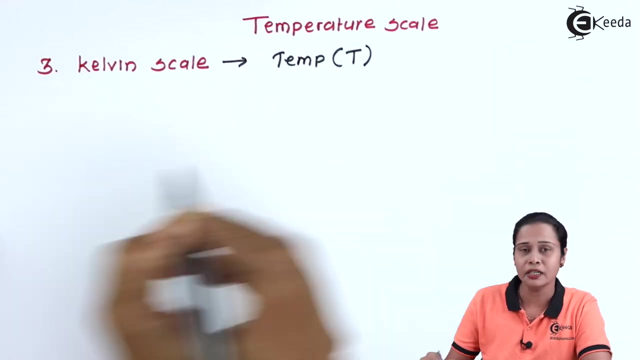 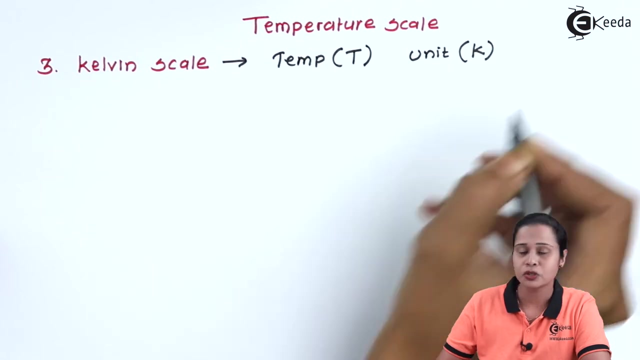 Kelvin scale is designed by scientist Kelvin. that is why it is called as Kelvin scale. Now, here temperature is denoted by capital T. In Kelvin scale, temperature is denoted by capital T, and the unit of temperature here is capital K, So that capital K is nothing but Kelvins. 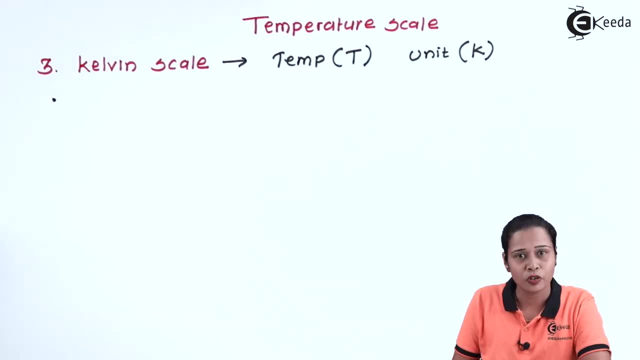 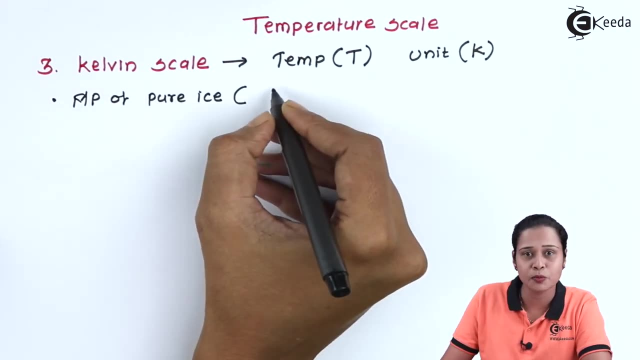 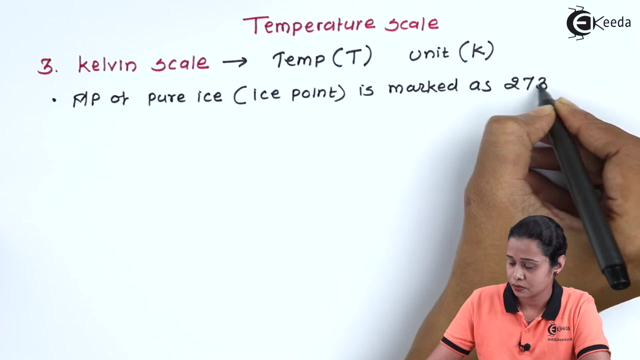 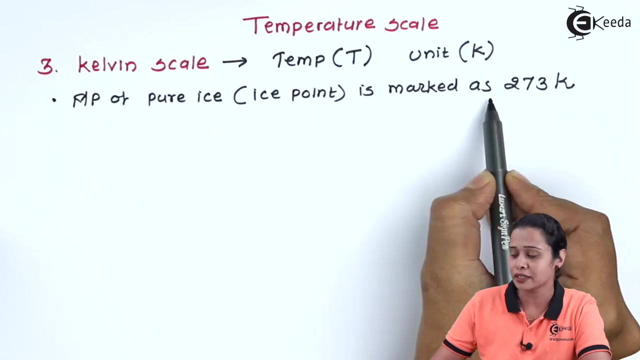 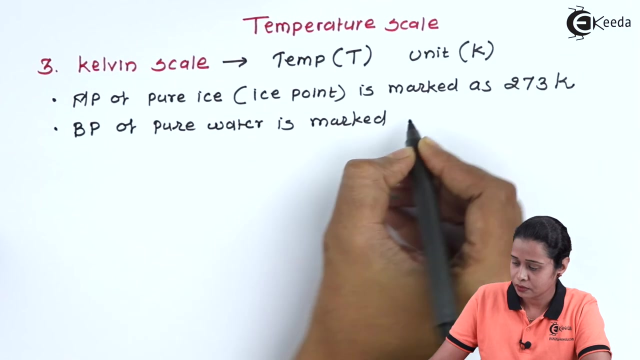 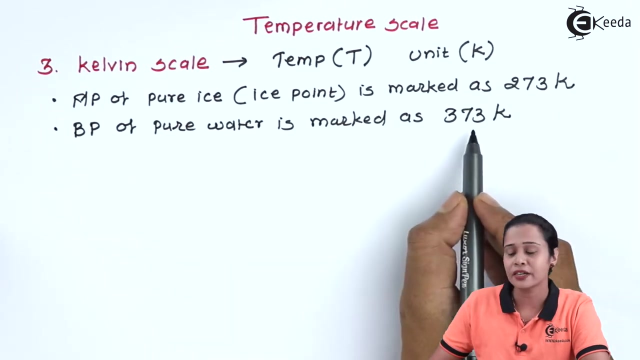 Now here, first point, that is melting point of pure ice, That is ice point. So here, melting point of pure ice, that is ice point, is marked as 273 Kelvins. Now second point, that is boiling point of pure water. Here boiling point of pure water is marked as 373 Kelvins. 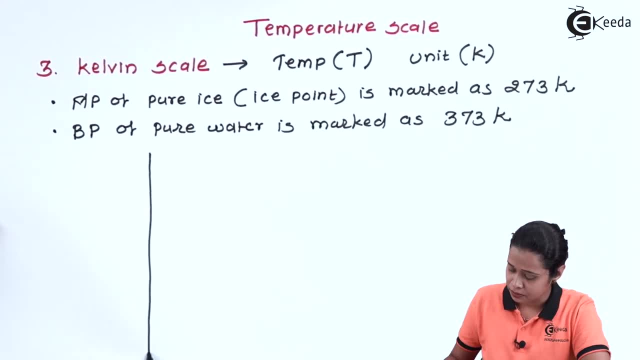 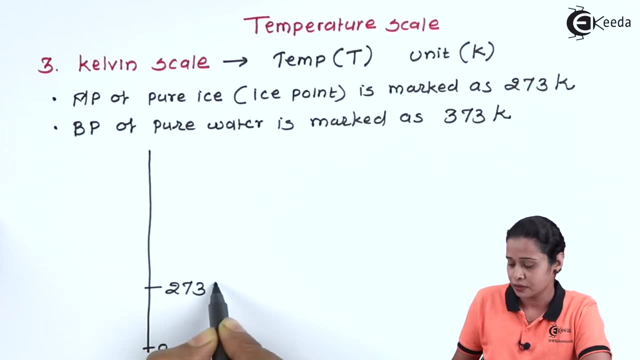 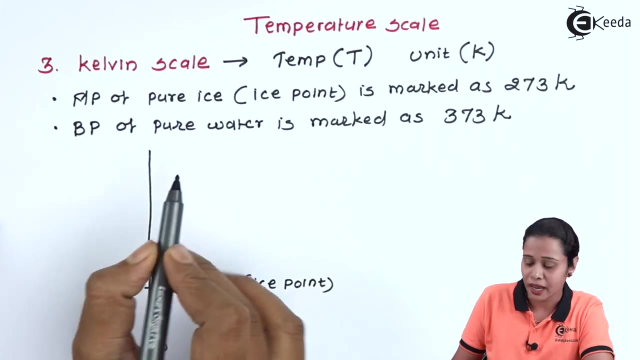 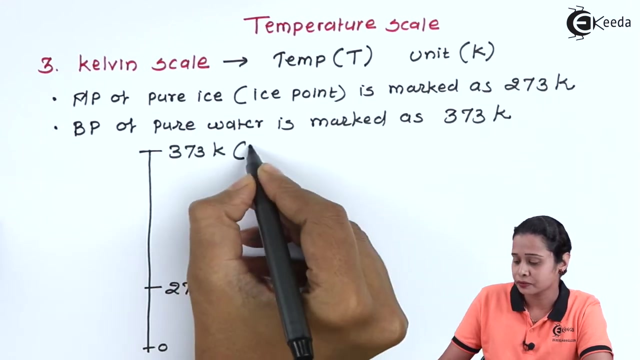 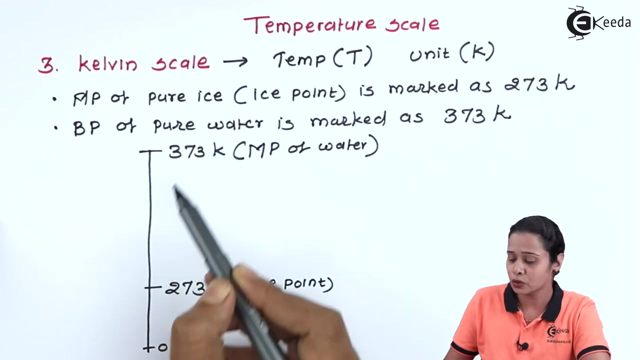 Now we will see scale. It will start from 0, but here, at 273 Kelvins, that is the ice point, And at 373 Kelvins We will say it is melting point of the water. Now this scale from 273 to 373 is divided into 100 equal parts.